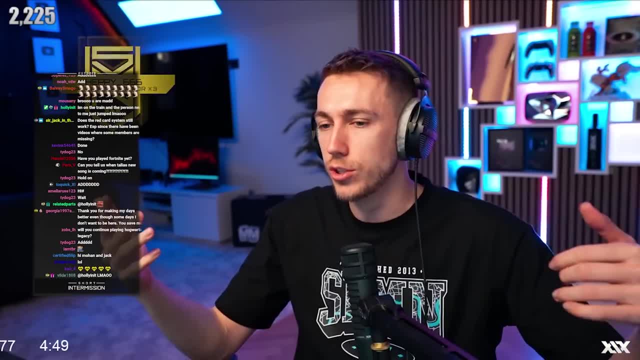 you get a red card, And when you get a red card you lose the video. So Josh could do 20 videos and I do 10, but if he gets 15 red cards, he's technically only done five videos, even though. 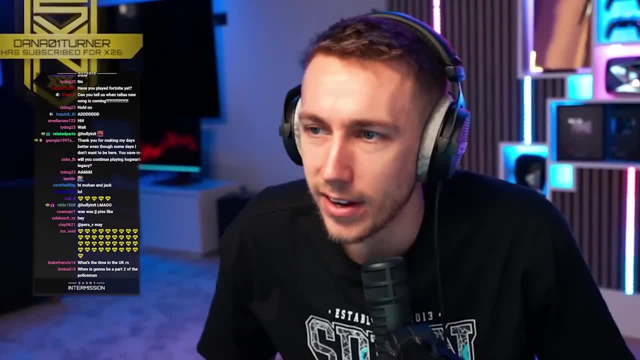 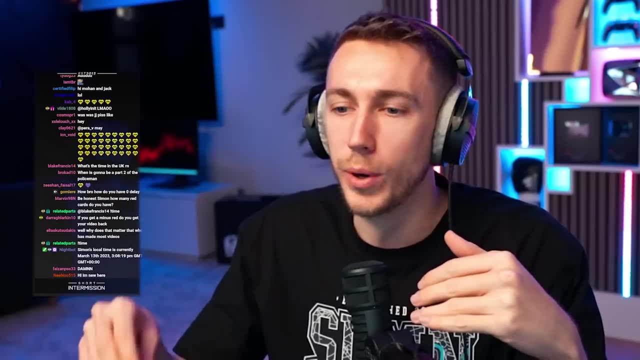 he's done a lot more work. he's then lost 15 of them, And then we'd always try to keep it level, So like if Josh had five videos not red carded and I had 10, we would go right. what's the next? 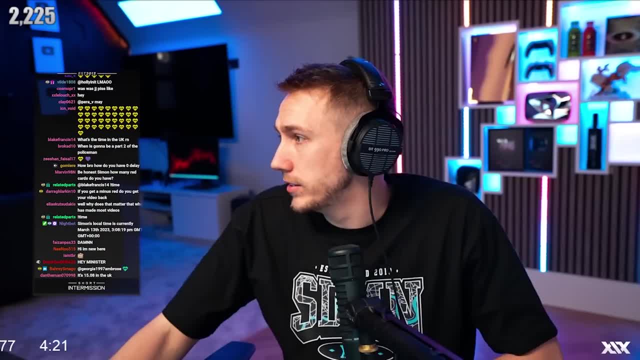 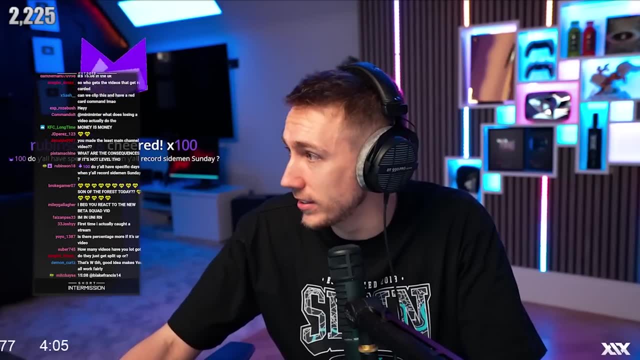 video. Josh, you have to take that. But yeah, me and Josh both have four red cards. Ethan has seven and a half red cards, Harry has eight, Vic and Toby both have 10 and a half red cards And JJ has like 11,, 12,, 13,, 14,, 15,, 16 and a half. I'm catching up, though, in terms of videos. 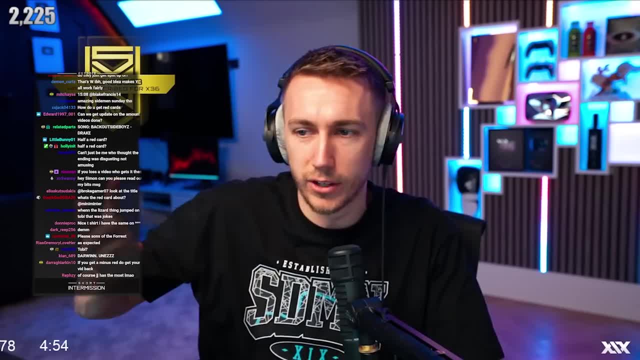 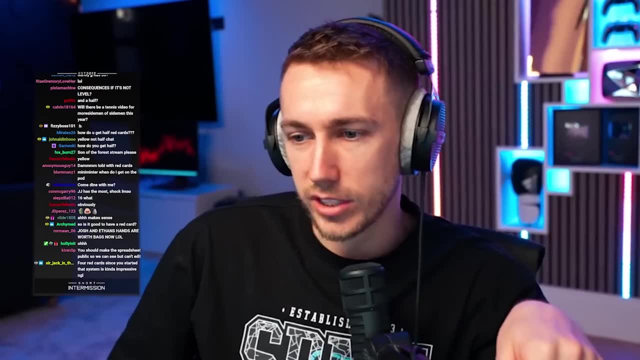 because you guys got to remember, I did a half a red card as a yellow card. as in they have seven and a half, So like the half is a yellow card. So if they get one more yellow card they've got a red card. So is it good to have a red card? No, no, no, no, no, no. Basically, 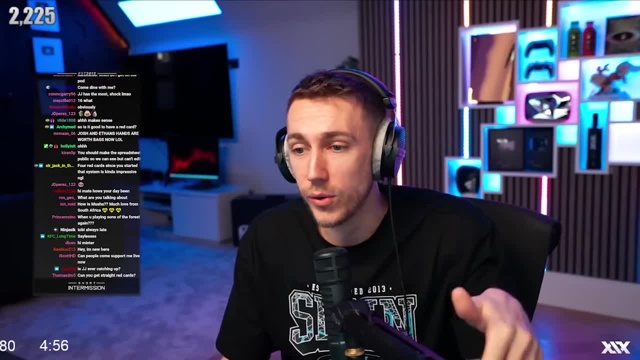 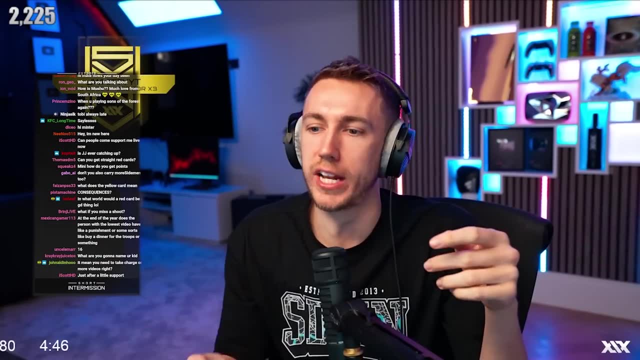 for example, if I could do one video, can you get straight red cards? Yes, If you miss a shoot completely. So like if, if we do an online shoot and someone just sleeps through the entire thing, you get a red card. If you're late, yellow. 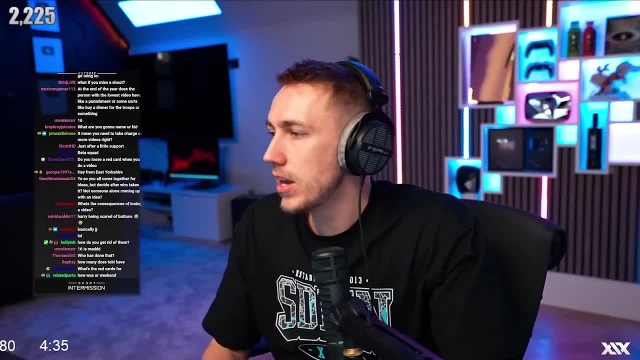 card. So yeah, we all. so yeah, we all come up with an idea. You know, we all came up with let's do this. Well, Beta Squad did it, but we have an idea. We go: let's do the try not to move. 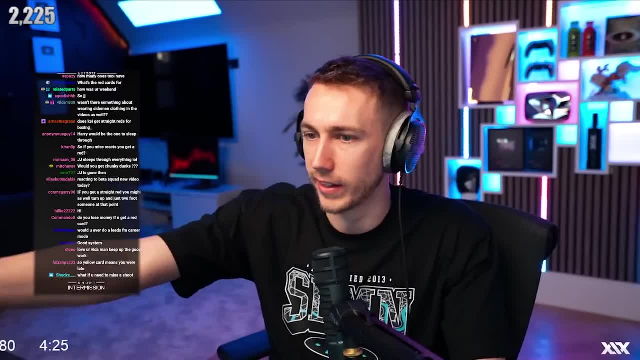 challenge: Who wants to take it? Someone says I'll take it. Or we look at the list: Who's got the least? You do it. So then that person will take it, and that's how it works. What if you need? 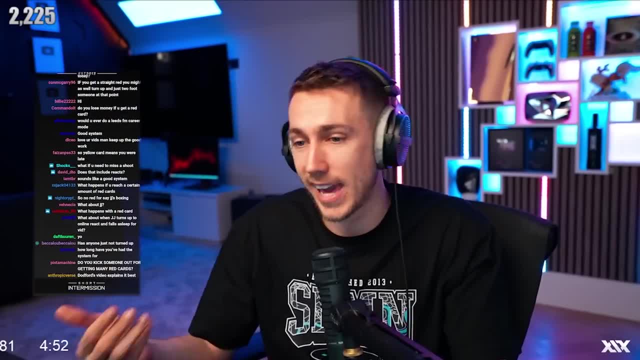 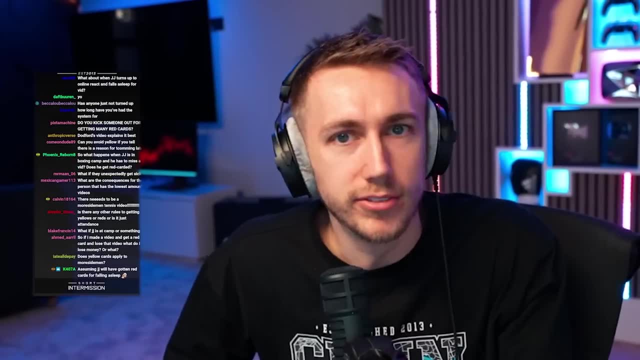 is reasonable, Not a red card. Like JJ in camp doesn't get a red card if he misses Cause, it's like you can't expect him to If. if Ethan has to take care of Olive, it's not a red card. Yeah. 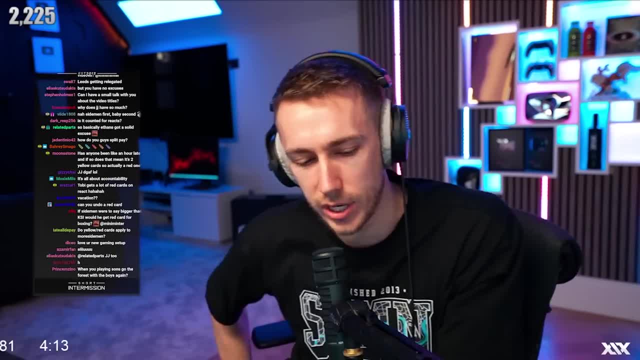 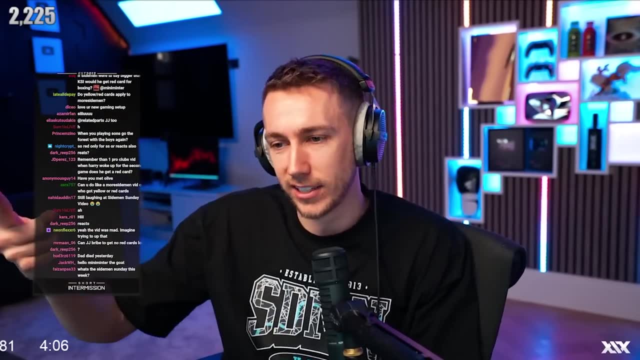 It's all about accountability. No you, if you're an hour late, you still get a yellow. It's half an hour later, Cause if you're literally 10 seconds late to a shoot- like 30 minutes and 10 seconds- you get a yellow. but the red cards or yellow cards are sometimes voted So like. 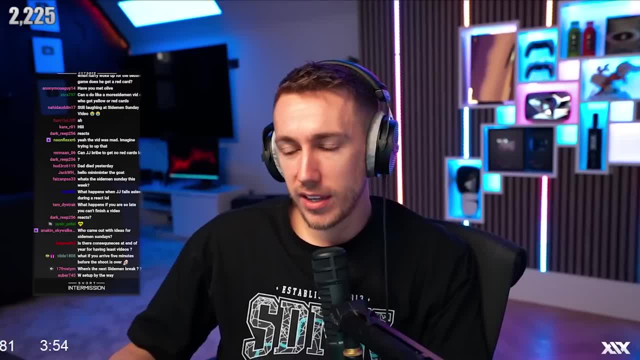 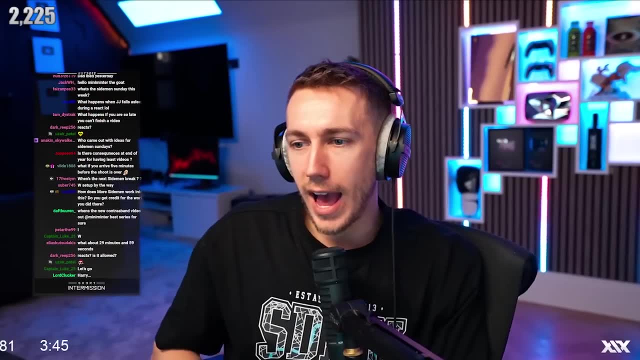 I'm trying to think of a situation. Someone's game might not work And if we can tell it's not their fault, we'll have a vote and say: yeah, you, you don't get yellow. Uh, how does more sidemen work into this? Do you get credit? 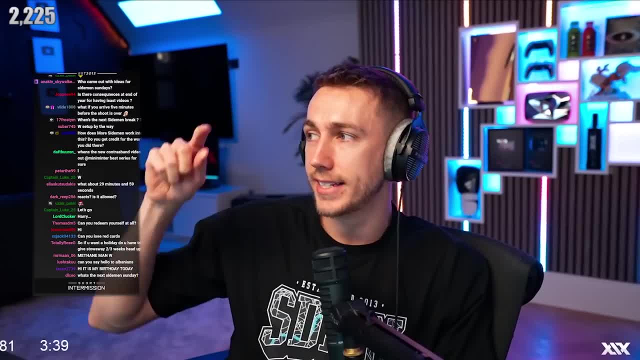 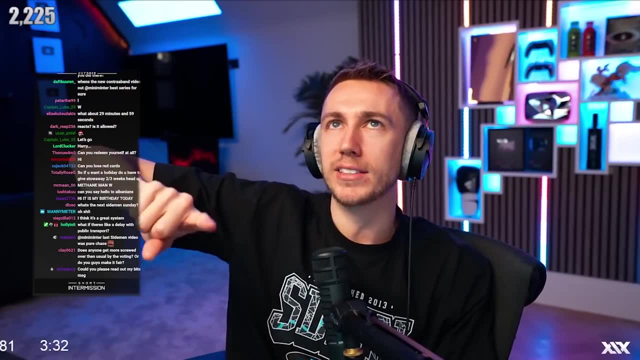 for the work you did there. No, So the way it worked was I did more sidemen. Um, I would basically just organize the videos with a couple other people. Well, we didn't really have as many people back then to help organize. I would organize most of the videos, And then what if? 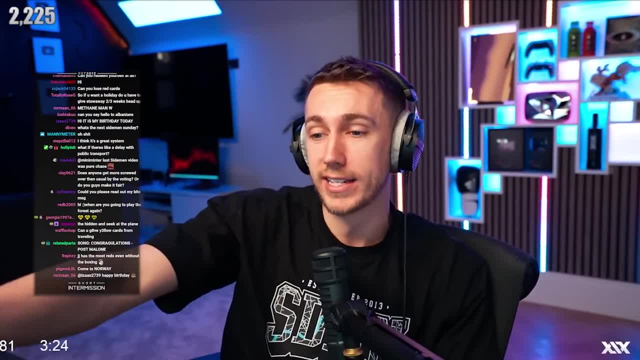 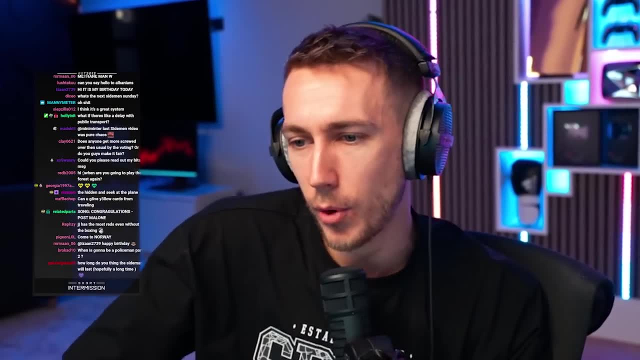 there's a delay with public transport, That's your fault. We allow 30 minutes for that delay Cause. realistically, if it's at 1 PM, you're aiming for 1 PM, So you have half an hour for delays, because you should be there on time or early, not late. Those more Simon videos I didn't. 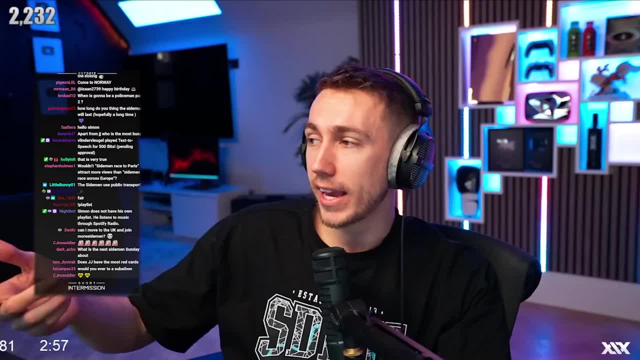 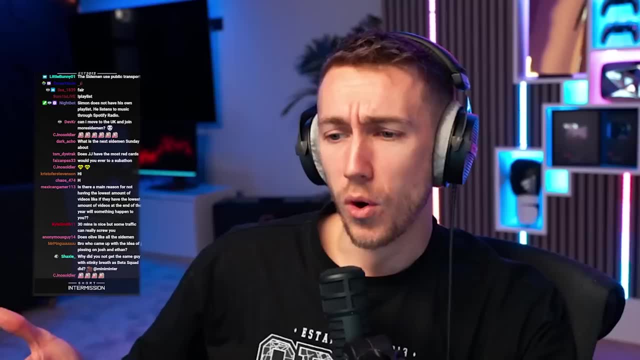 do main channel, So I just wasn't included in the road So I could still get a yellow card, still get a red card, but I don't really know how it worked with that. But at the same time I didn't get any, or I got like one or two. You're the one who tells the editor to use. 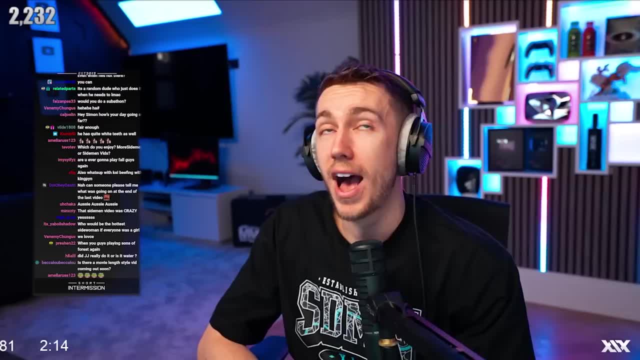 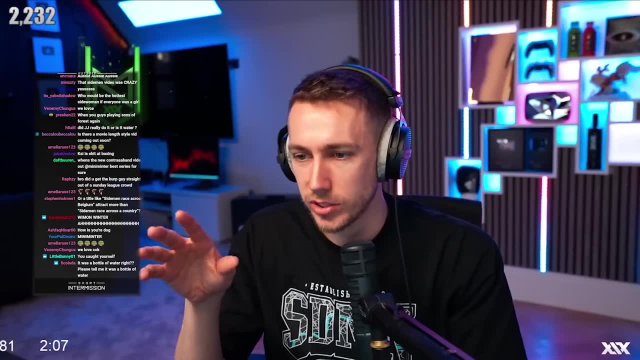 JJ and the thumbnail No. So more Sidemen, I haven't. I organized the real life videos. Now I go through them and, like you know, edit them slightly in terms of getting the questions. So they'll, we'll hit, we'll find ideas and go all right, this one Cool, And then I'll get sent. 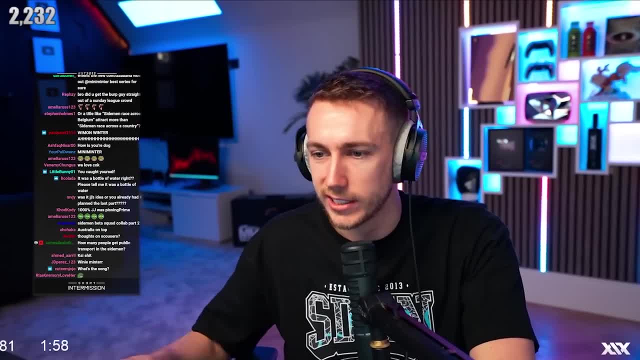 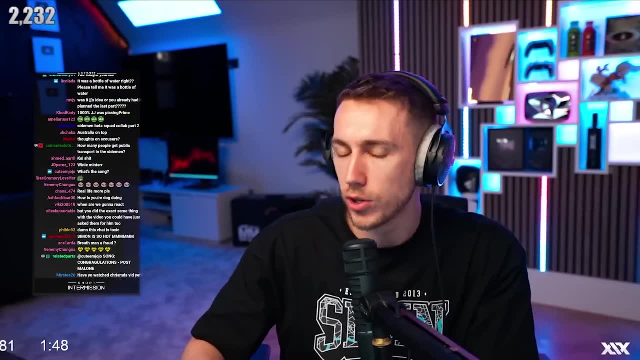 the questions to go like: get rid of this one, get rid of this one, get rid of this one. I'll change this, use this one, use this one, I'll do that. Hence why I ended up hosting them: because I've seen the questions, because I've worked on it, but I don't have to organize as much in terms of 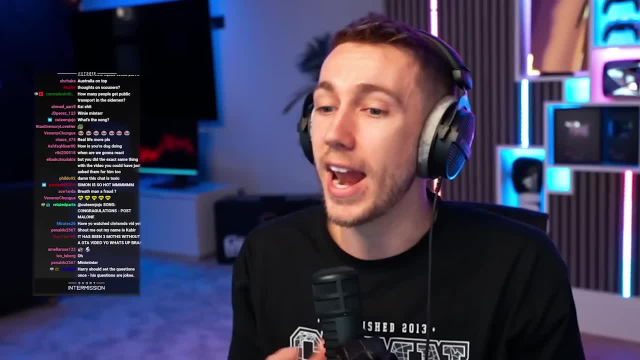 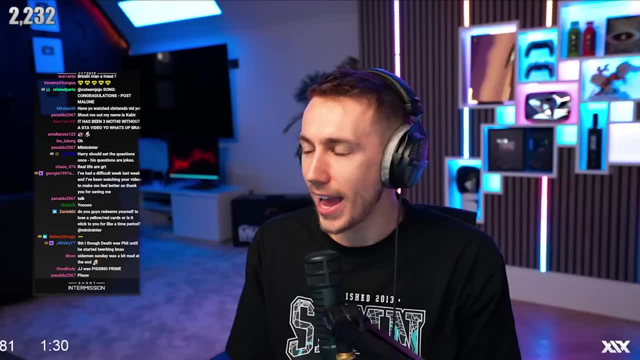 I don't come up with the well, not come up with the ideas, I organize the ideas anymore. So now I'm back on main channel And I mean the thing is I actually just like I like organizing videos, Like I actually find it fun to organize videos So realistically. 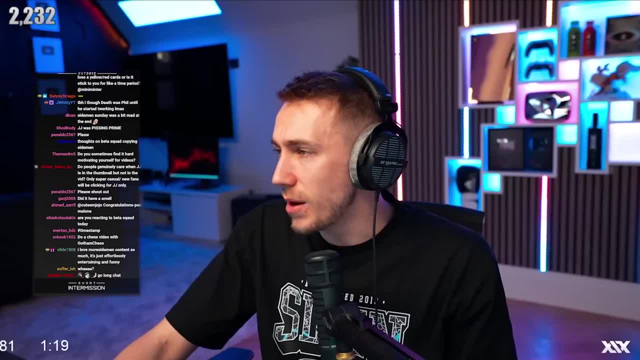 when I started this, when I, when I came back to the channel, I was on like I must've been on- like three videos and everyone else was on like 20.. So I'm catching up. They were going to just give me. 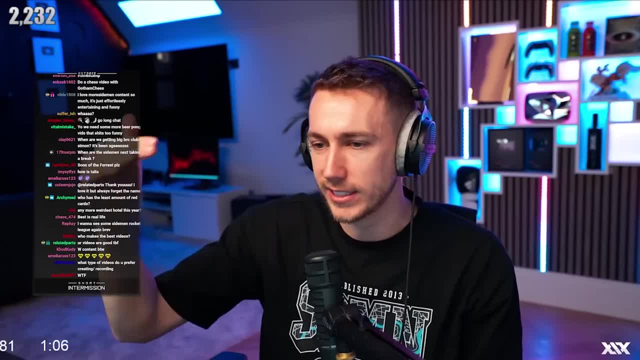 like a median and just go right. How much is everyone on? If someone's on like 15,, 16,, 17,, someone's on 20, they'll just go all right. you can have 16 and carry on. But I was like 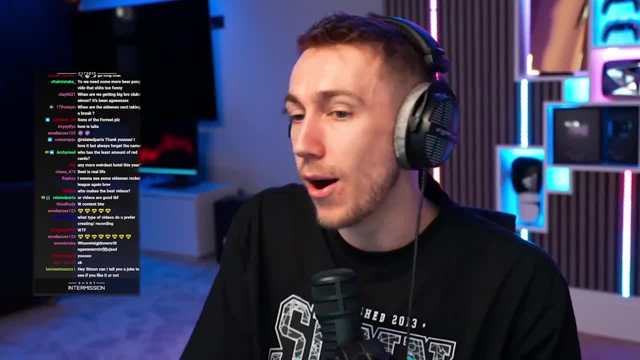 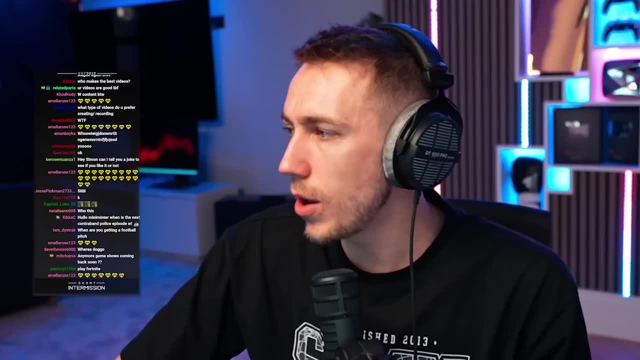 I don't really care enough to do that. So, um, I'm now. I have the least videos done. I've done 12.. The next lowest is Ethan on 21.. So my aim is: by the end of the year. I want to catch up. I'll probably still be lost, but I do want to catch up. Who comes up with more? 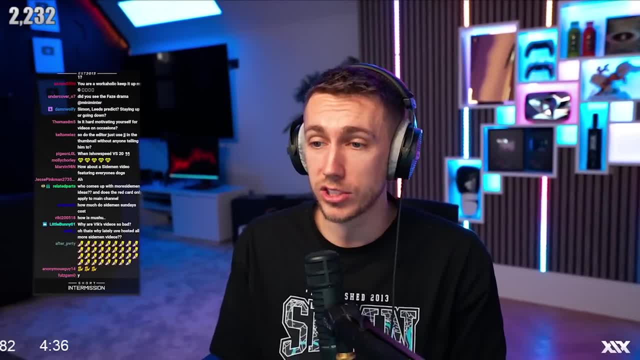 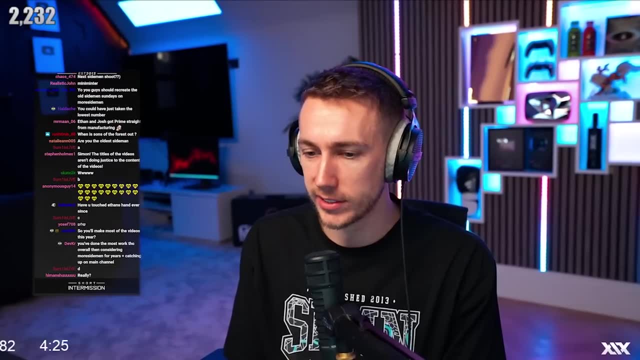 Simon ideas, and does the red card only apply to mainstream? No, So it applies to all of them. The ideas: We have a few people now that we've- we've now hired a load of people, So they'll then talk to us and say, Oh, mainly like they'll. I'll hear a lot of them and say, like, don't do this. 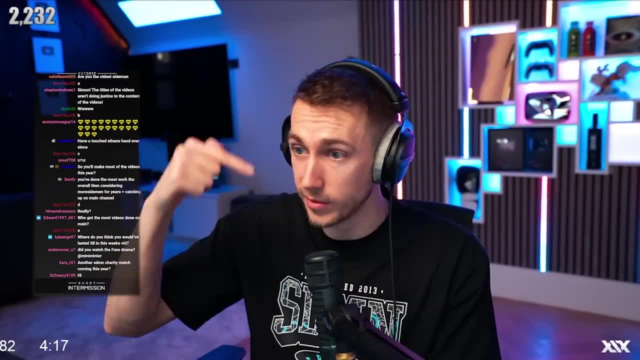 Don't do this, Use this, use this, use this. Then they'll send me the questions and I'll talk through the questions and get rid of some of them and do that, And then that's why I ended up posting it, Cause I've seen the questions and work through them. 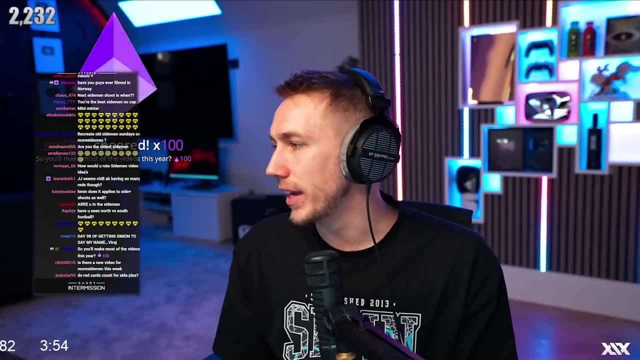 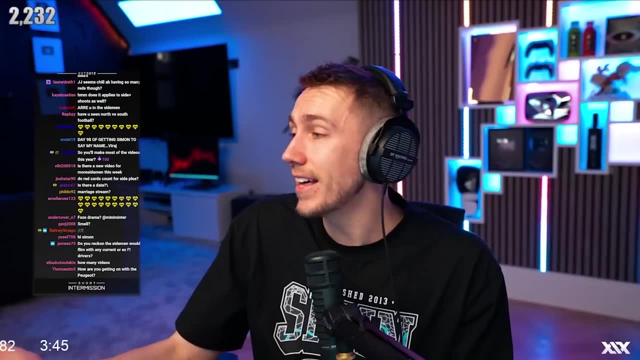 and stuff. JJ seems chill about having so many red cards, though I mean he is, but it's cause he takes. he does take a lot of videos. He's taken the most videos. Just he loses a little bit. So you'll make the most videos this year. Yeah, That's probably what happened, But as I 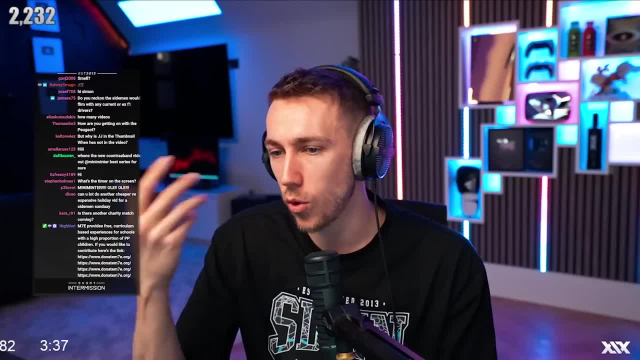 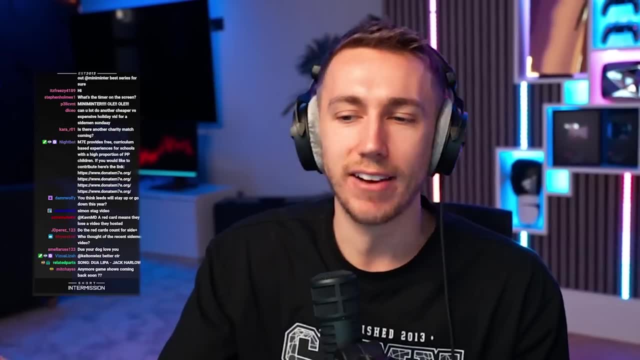 said I like doing it, Like I actually really enjoy hosting videos and organizing videos. I actually said like I think I would happily what I kind of want to do for when I eventually have a kid. when I eventually have a kid, obviously you know how normally you would. 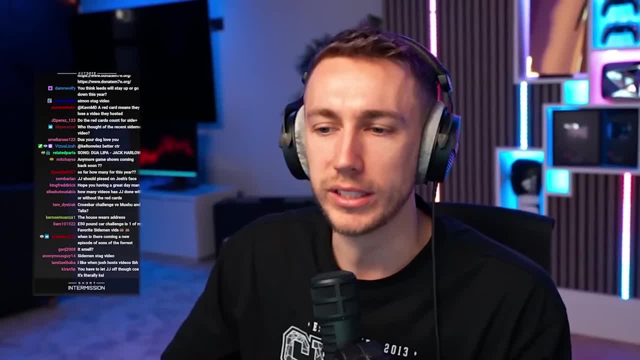 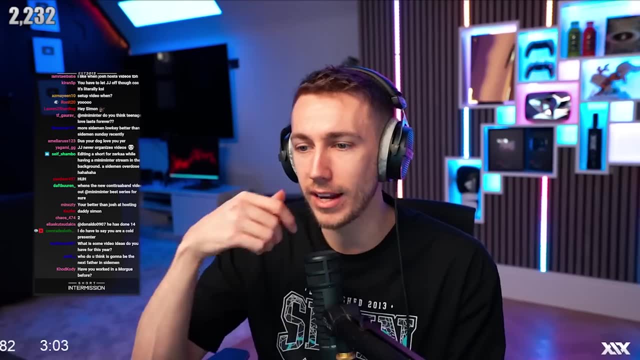 take you have like um, like a couple of weeks off or whatever. I would love to have more time off, but organize all the videos in that. I would love to do that Suggestion for future hide and seeks. Don't count them on your tallies Now what we decided about hide and seeks. hide and seeks. 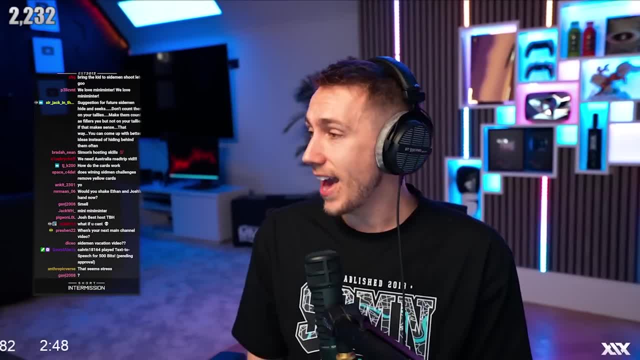 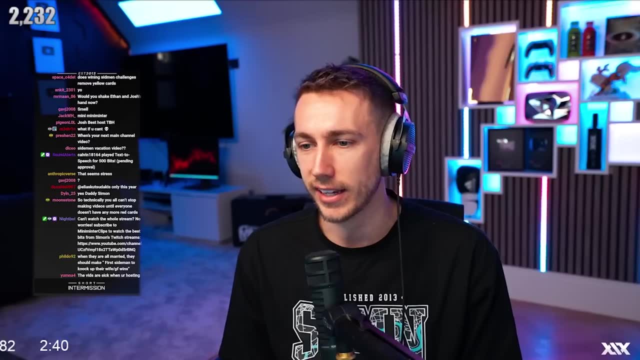 actually changed recently. Hide and seeks actually changed recently And we basically we've always done: if you've got a hide and seek, it's just the, it's just the easiest video to host, to sort, Like in Europe. for example, the one we did that was Vic's video. You literally just you have the. 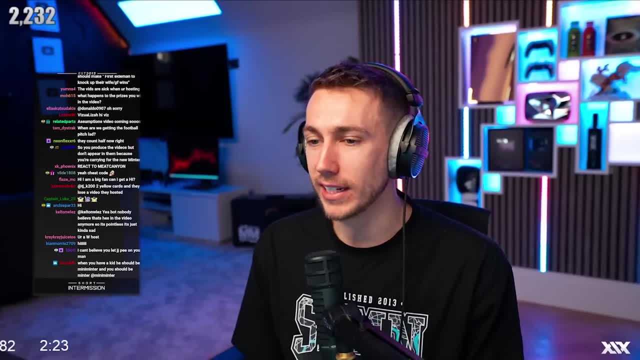 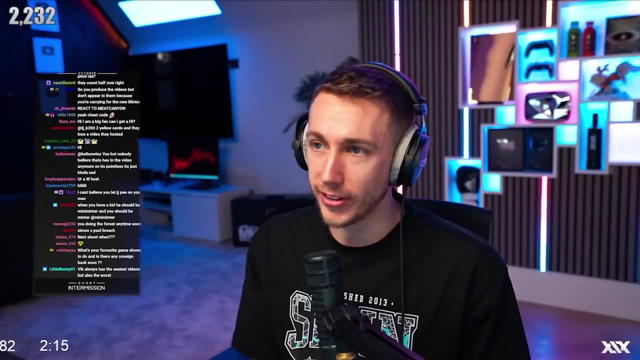 location. That was it. That was the video. Like the day before I said, do we not have outfits or anything? And then he organized outfits the last day, Like it's so easy that. So what we've now decided is you get half a video for hide and seeks and whoever's hosting them gets uh, hosting. 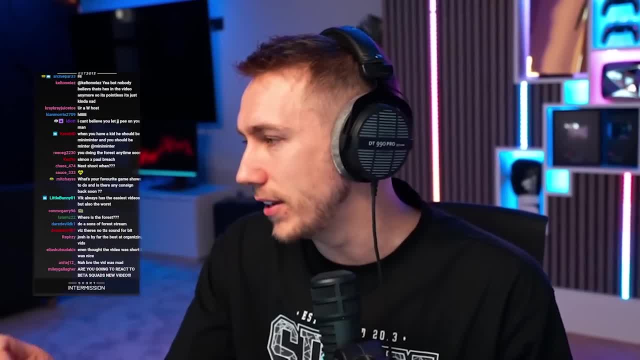 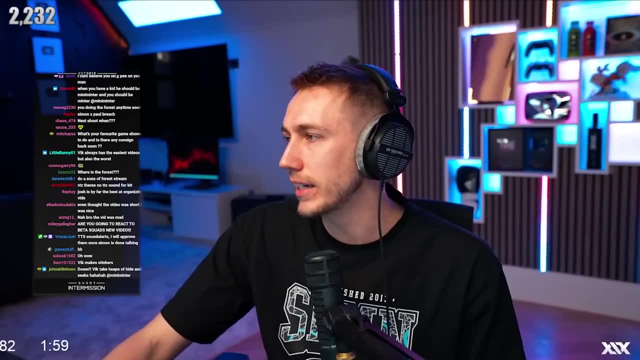 whoever's seeking gets half a video, which is kind of peak for JJ, because we actually figured out who has the most. uh, like we figured out that basically JJ has seeped way more than anyone. Will you do more wild forfeits? So people take the video. 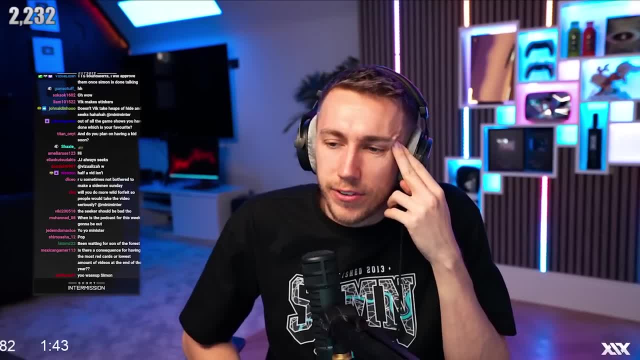 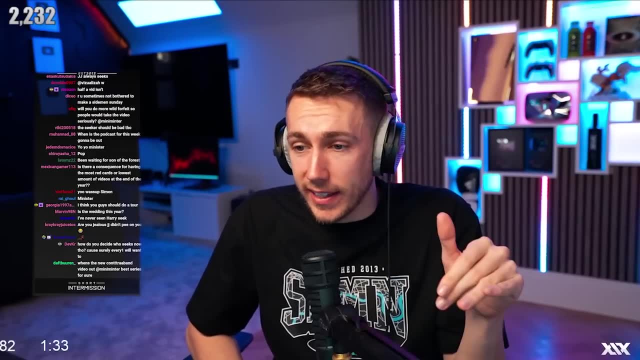 seriously? No, because I don't think there's that much. There's not. there's less fun when it's that serious, Like there's a lot less fun when the video has to be taken seriously. It's why I don't think anything. Yeah, Anything that's like a genuine race, like a real race. Isn't that fun? 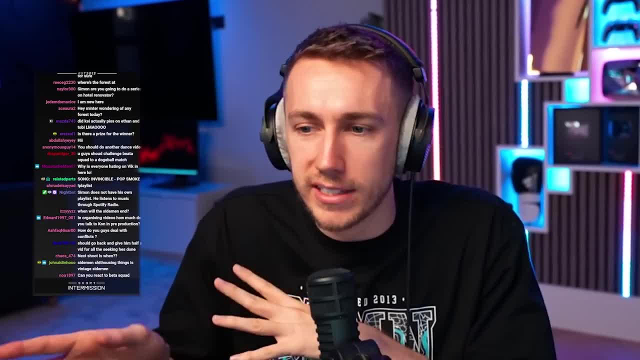 I'm not talking about a race across the country. I'm not talking about like a race from the desert. I'm talking more like put us in a car and it's just like a race. You won't get people talking because they'll just want to win. 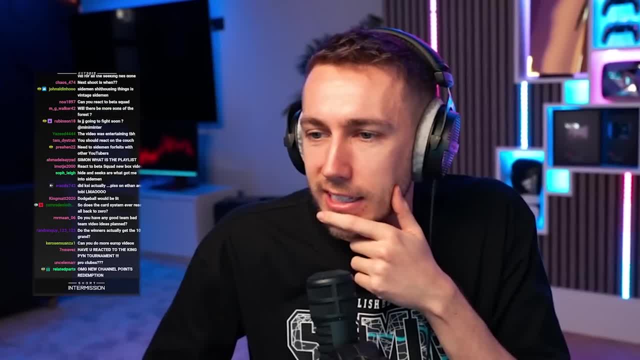 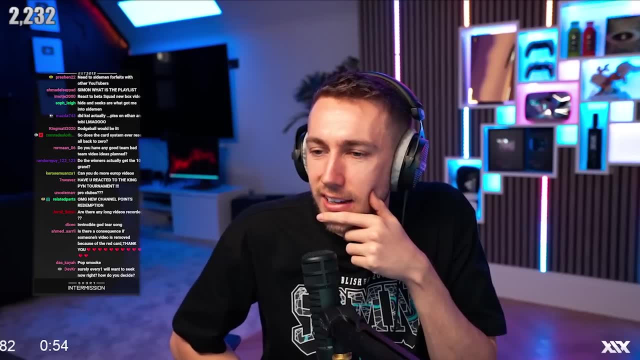 Now that I've said about the um, now that I've said about the hide and seeks, it shouldn't really happen. I don't know if Josh is still here. We shouldn't really have that system because it is unfair to JJ and everyone will say, yeah, I'll seek And I don't have to put in a good 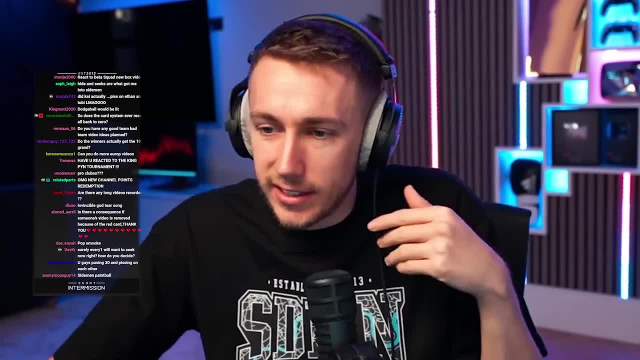 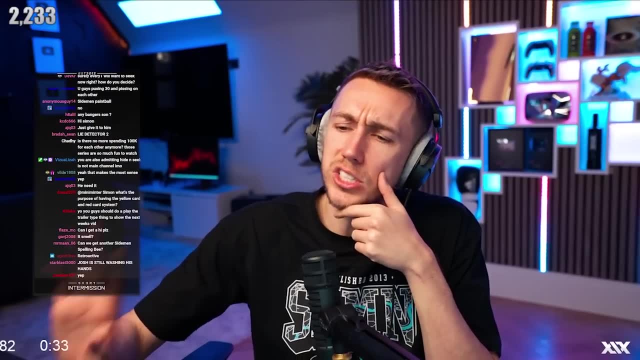 shift. I just it should just be. if you take the video, you have to see. I think that's, I think that's the fair way. If you take the video, you see you are also meeting. hindsight is not main channel. No, cause, we're still having a full, like a full, video. We're just saying that whoever's. 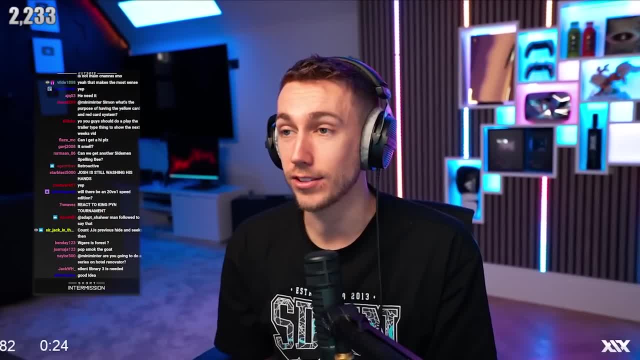 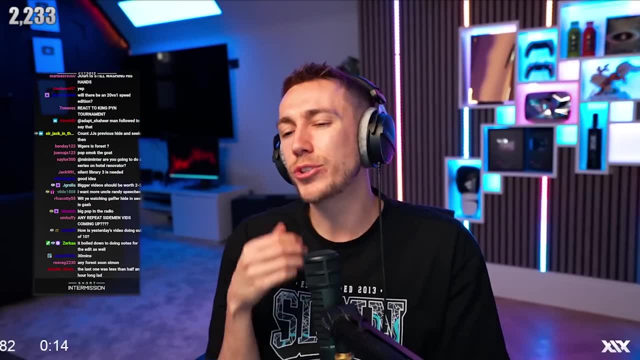 seeking is doing the hard work, Like seeking in the hide and seek is long. Like it is long in certain places, Like the, the boiled down to doing notes for the edit as well. True, But now I'm thinking about it, I'm like I think 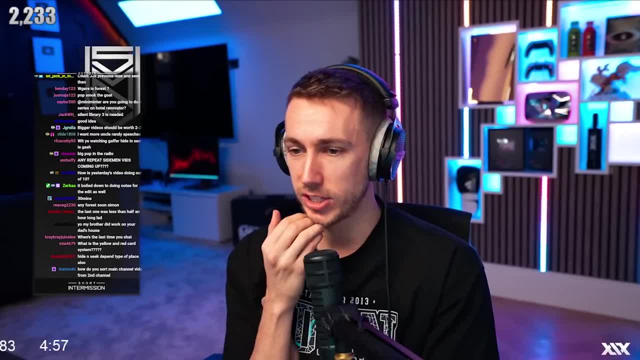 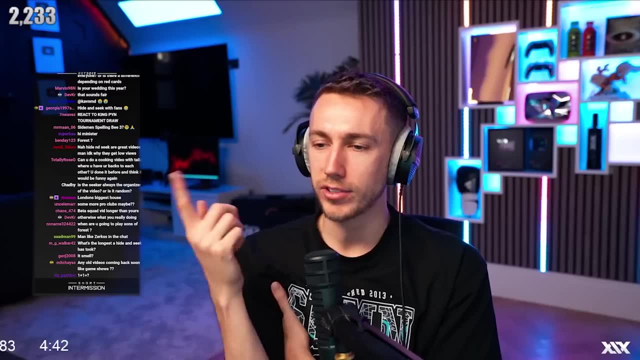 you just have to host. If you're taking the video, I think you just have to host. That sounds fair. Yeah, Cause, realistically it's like if you're taking, I could take every hide and seek and just go: all right, JJ, you have to, you have to seek. He takes half a video, He does the long part, He. 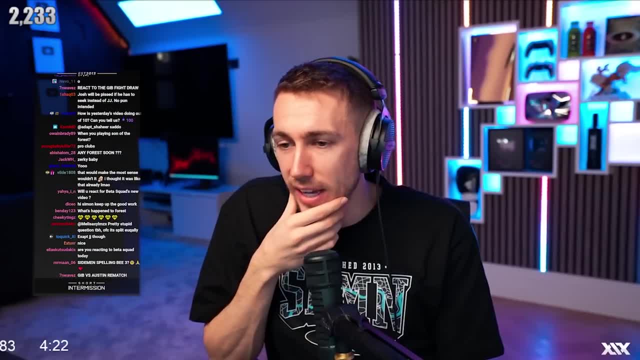 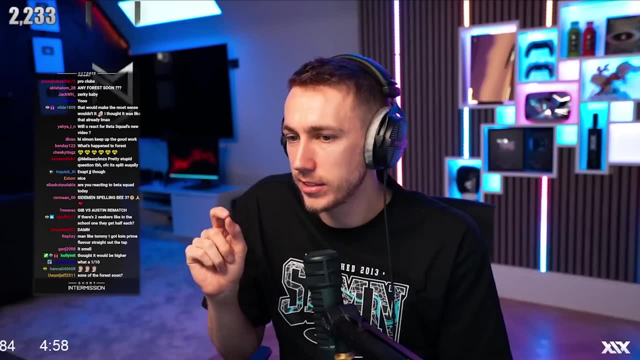 has to watch the edit and stuff. That would make the most sense, Wouldn't it? I thought it was like that already, But no, we cause JJ. I think JJ is the most content seeking. JJ is the most content seeking by a mile. But I understand that when you go to start, like when you start going to such large 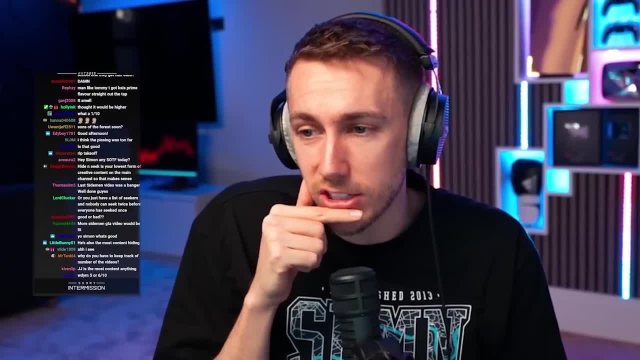 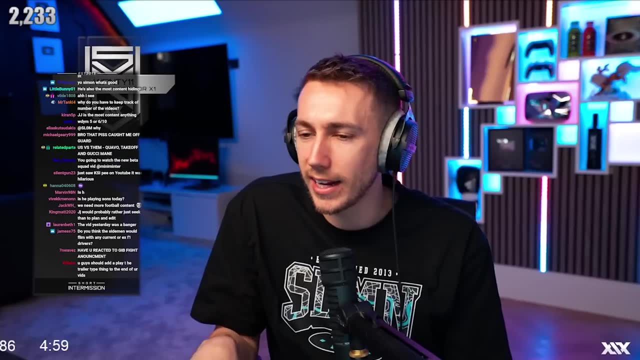 locations. it is long as hell, Or you just have a list of seekers. When I'm saying this- right, I'm talking- I think JJ has seeked like 11 times. I think, like I want to say: like me, me, Josh. 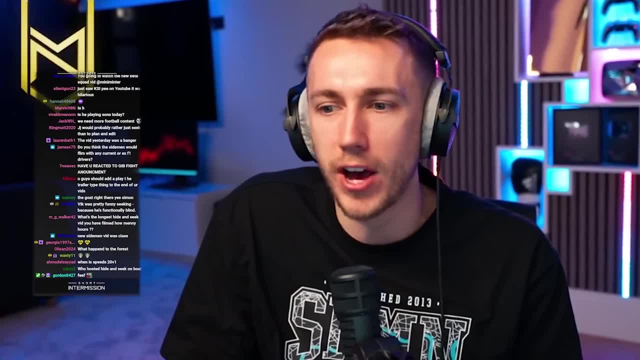 Harry, I think are all like somewhere between like five and eight, And then I think Toby, Vic and and Ethan are like three. 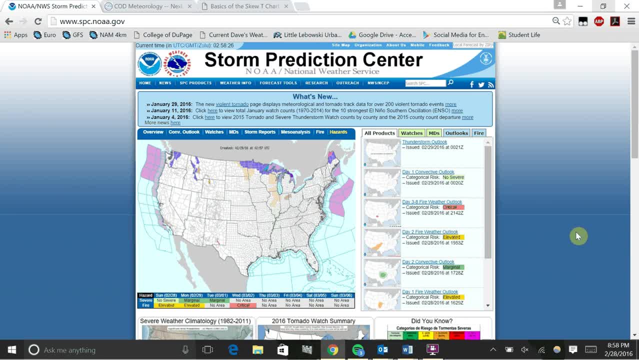 Hello, my name is Matthew Deer and I'm here to give you some basic instructions on how to find and utilize SCU-T plots for severe weather forecasting. Basically, a SCU-T plot is a representation of the vertical profile of the atmosphere at a specific geographic place, like a city, for example. 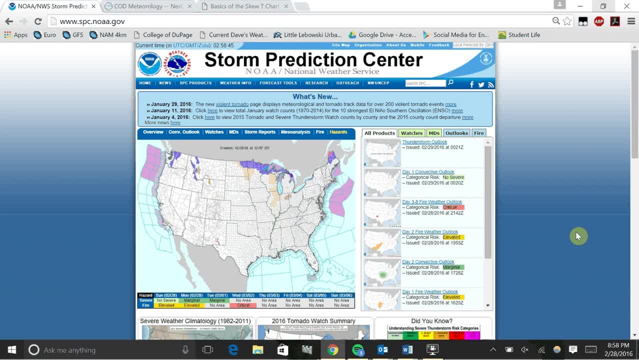 One good example is that every National Weather Service station across a country launches a weather balloon at 12Z and 0Z every day. Those are Zulu times, That's for central time. like I'm in Norman Oklahoma, It's minus 6 hours, so at 6 am and 6 pm every day they launch these weather balloons. 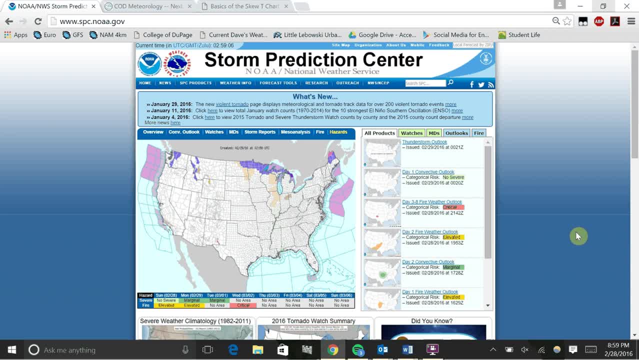 And the weather balloons make what's called a sounding of the atmosphere. It records the temperature, dew point, the winds and it publishes them on the Storm Prediction Center website which we're at right now- Storm Prediction Center. It publishes them in what's called a SCU-T format. 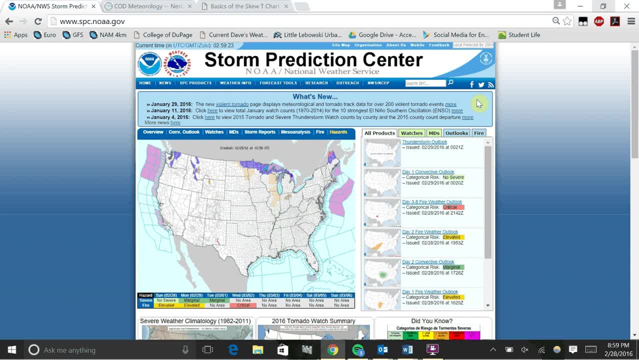 Now how to find the observed SCU-Ts on the Storm Prediction Center website. it's just spcnoaagov. You go to Forecasting Tools and Observed Sounding Analysis right here. Now that'll take you to the archive.